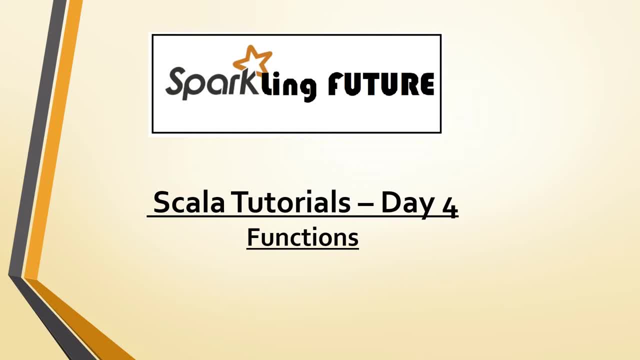 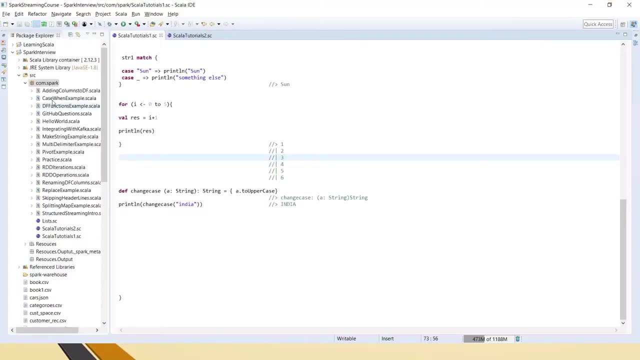 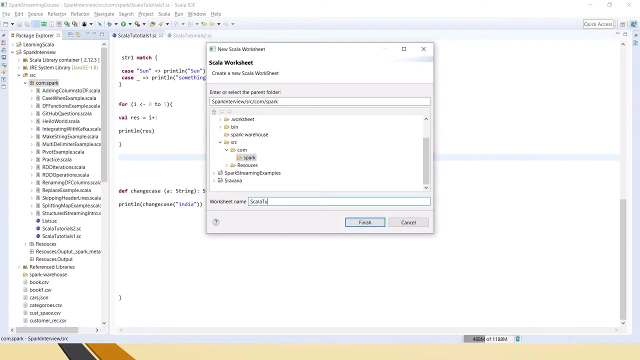 as parameter or even return them from functions. So today let's see how to define a function, how to call it and how many like. how can we pass types of functions and how can we pass variables, how can we pass functions- all these things we will see in today's video. So let's create a new Scala worksheet. I'll name them as Scala 3L3.. 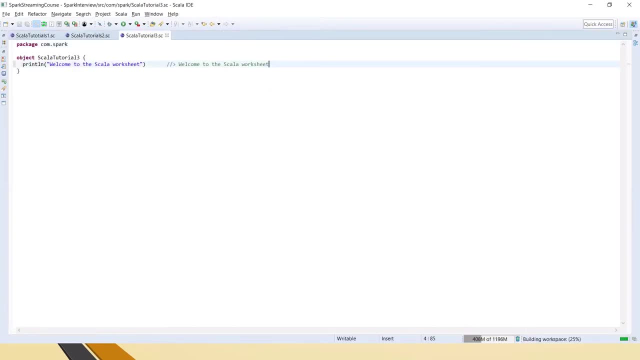 So first we will see the definition of the function. Def is the keyword for defining a function, then function name, inside the parenthesis parameters Return type equal to and the definition, the function body. Okay, So if you see here, equal to, this is the main important thing in the Scala function. So this is the definition. This is how we will define the functions in Scala. So let's start with a very simple example. Okay, 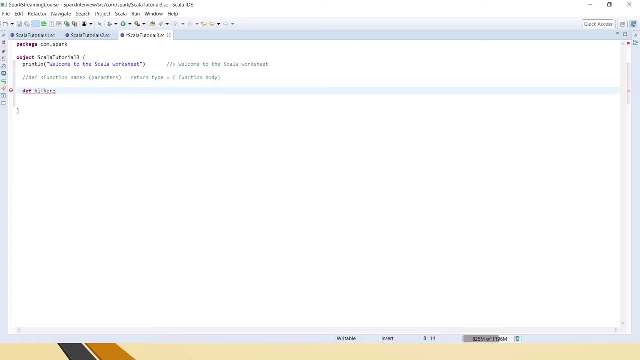 definition: Hi there, Okay, Because usually people start with hello world right. So just like that, Hi there And sorry. And if you see, inside the print lm, I'm calling this function definition here This is how we will define a function Definition is a keyword: Hi there is the function name. It doesn't have any input parameters. No return type is mentioned, So automatically it will take it as a unit here in the like in the. 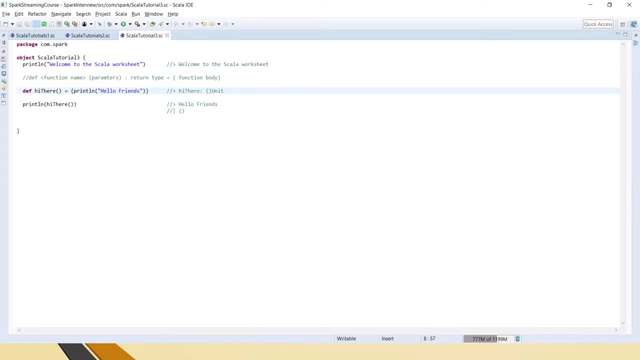 Answer section you can see what type it has considered And here you can see that unit means any type. any type is called, the unit is considered. And when I say print lm and hi there, it went inside this function and it has printed. Hello friends, You can see here. So this is how we will declare function in Scala. So let's look into some some how to do some of two integers. Okay. 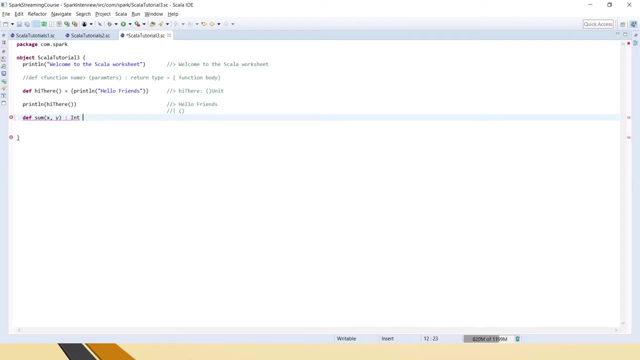 x comma y, and we'll say that return type is also int, equal to, and inside the braces we'll give it as x plus y, which means it will return x plus y. Okay, x is integer, y is integer and y- it has insisted me- is specifically giving the return type. So, which means I should mention the types here so that I can. I will not be able to send a string again, because the return type should be a int here, But after this operation it will become a int. because of that reason only, it has given the error. So now let's print. 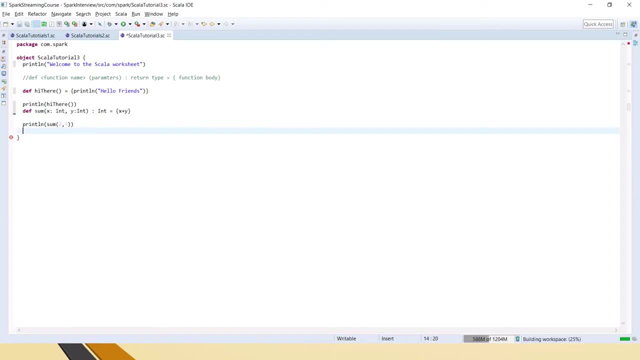 Sum of two comma three, You can see that five. So this equal to is used as a assignment operator here, which means after executing this, The answer is assigned. Okay. So that is the meaning: assigning function to some expression. This to this expression we are assigning this function, Okay. 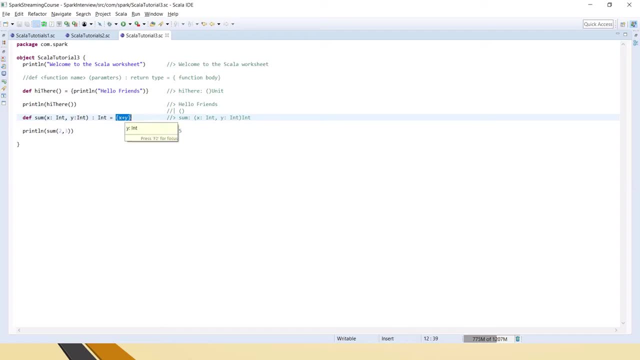 So So this: this is how we will work with the functions in Scala. So let's do getting a square Square of the Given integer X into x, Capital I And return type is int, So println Square of four. 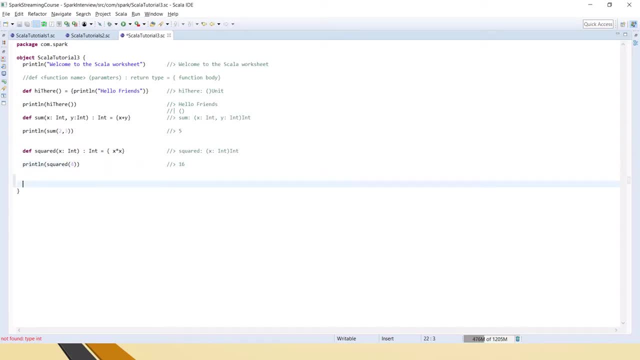 And Four into four equal to six. the square of four equal to six. So this is how we will write the functions And, as we say, as I said, functions can take functions as input parameters. So let's create another function called And func. 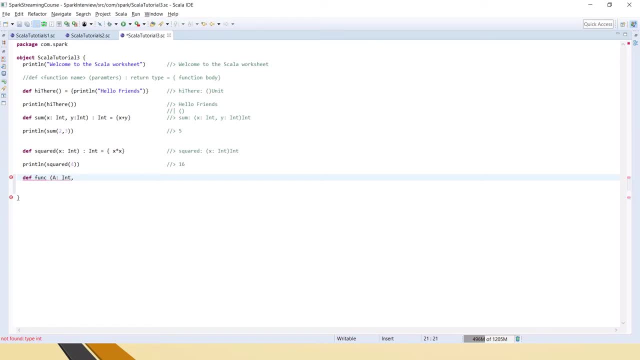 And A small One: integer I'm taking And second one I'm taking it as a function. So if you see here the declaration For normal variable will give like this, for if you are passing a function You will do like this means that function. 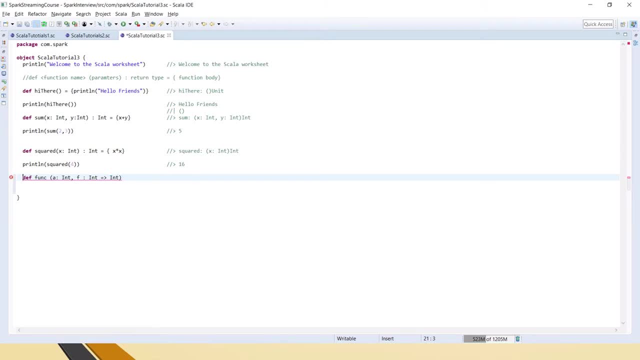 Will take integer parameter Return, say int. This is a meaning of this Line, And then This overall Return type is int. For this function, For this function also, we have to give the return type right. So That is the one. 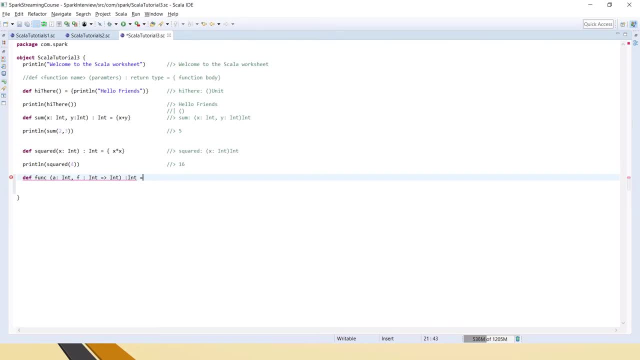 And Equal to. In multiple lines also we can write like that: Anything is fine, So f of A Means. Here We are passing one integer and one function And that to that function itself. we are passing this function as input. 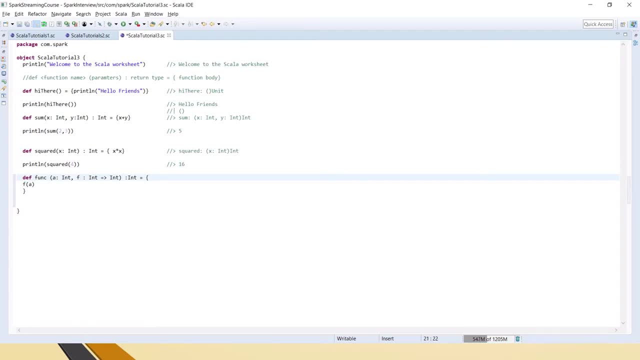 Okay, So now We are passing One Integer And one function, And that to that function itself. We are passing this function as input. Okay, So Now Let's say Some result: Okay, Equal to Fun. 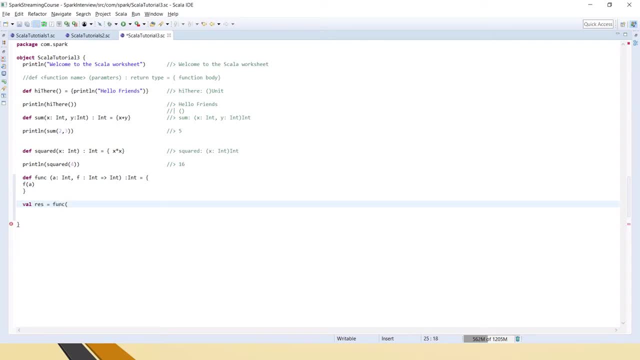 This function. Okay, To this function We have to pass two parameters. So Let's say five And Squared. Okay. So This squared is this function. So It has two parameters: One is integer, Another one is a function type. 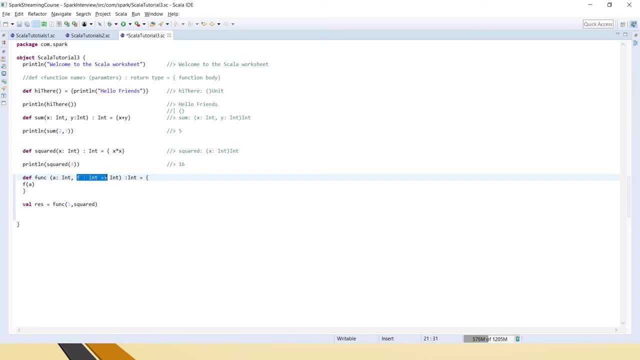 For the integer, I am passing five, And for the function, I am passing this Squared Function. Okay, So I am passing this Squared Function. Now Let's print this Result. So It should. 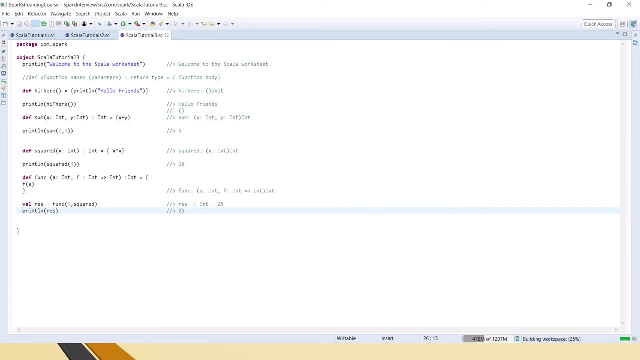 Give Twenty five, Five Into Five, Twenty five. So You Understood This concept Right, Passing A function As input To another function. This is the Main Like Beauty Of Scala. 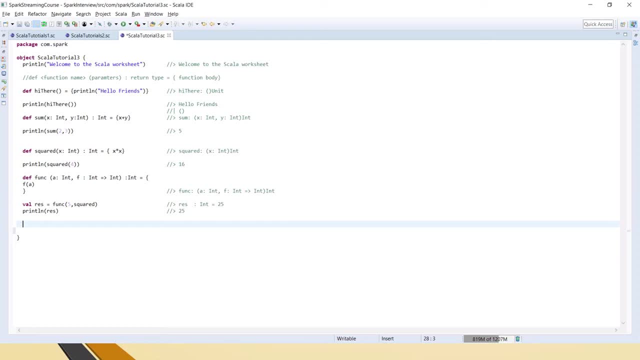 Okay, So Here, Instead Of Passing A function, We Can Directly Give The Body Also To This Function, Instead Of Here. We Said It Will Take. 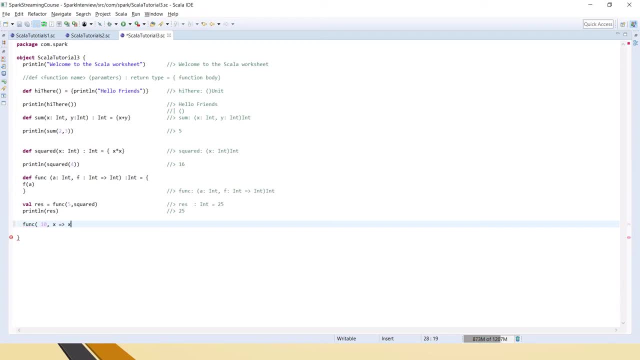 The Function As Argument Instead Of Calling Another Function. We Can Directly Pass Like This Entire Expression. We Can Pass Directly Okay And Usually For. 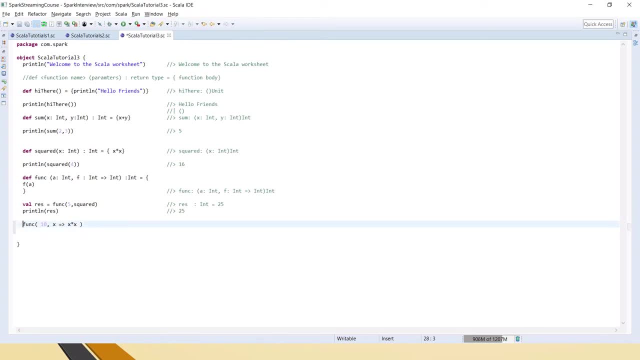 Any Short Expression For Anonymous Functions. We Can See Hundred, Ten Into Ten Hundred, So Like Directly. Also We Can Pass Like Some More Example: 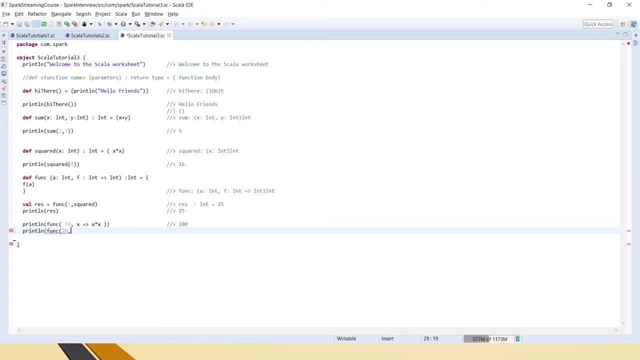 Also We Can Try. If You Feel This Is Very Simple, Okay, Got It Right, Then Also We Can. We Can Also Pass The Complex Expression. 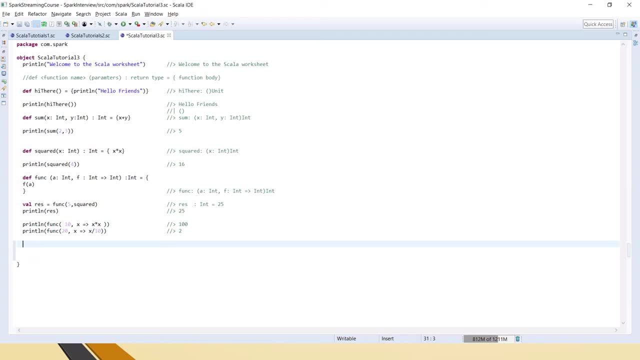 Inside This Braces. So Here It Says Very Simple. So Let's Say Five. And Next One Is Function. Right In The Function, We Will Say: 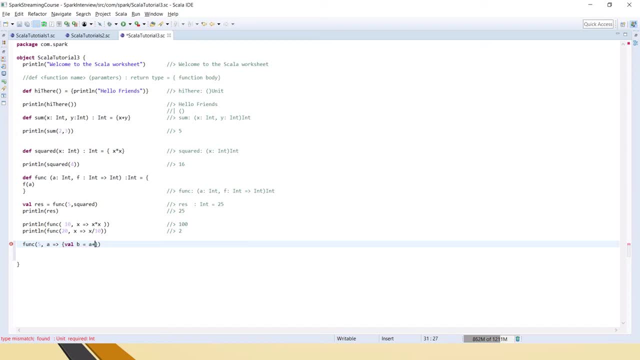 What We Will Do Is, First, We Will Take A Variable, As Val The Say Multiple Statement In A Single Line. You Have To Put A 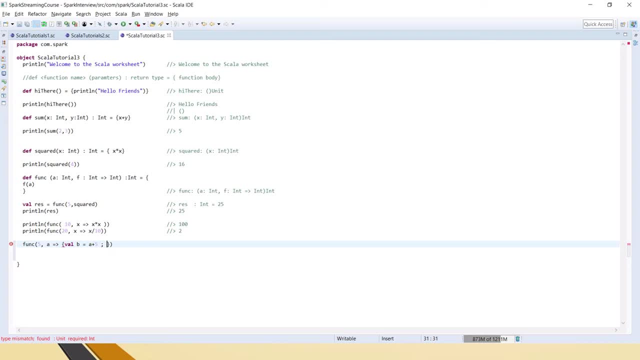 Semicolon For Separating The Lines, Because In Scala Each Line Is Considered As End Of Line. Now Let's Print This To See Whether. 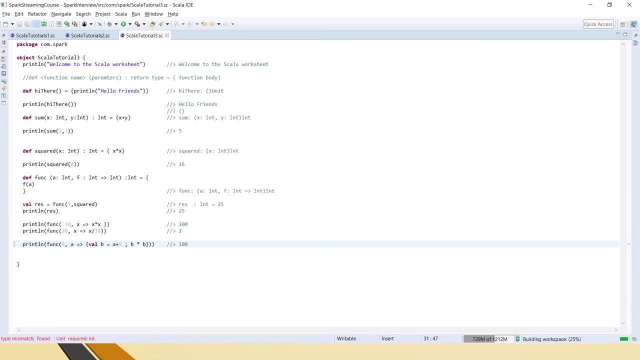 It Works Or Not. So This Five It Has Passed Here, Because To This A It Will Take The Input Parameter As Five. And Here We. 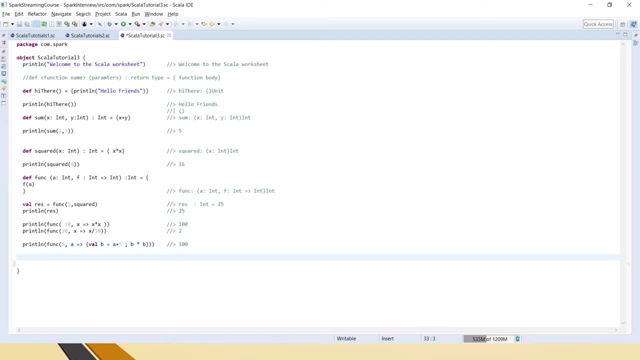 Are Multiplying Ten Into Ten, Equal To Hundred Clear No. So This Is How We Can Pass The Beautiful. I Mean To The What Is. 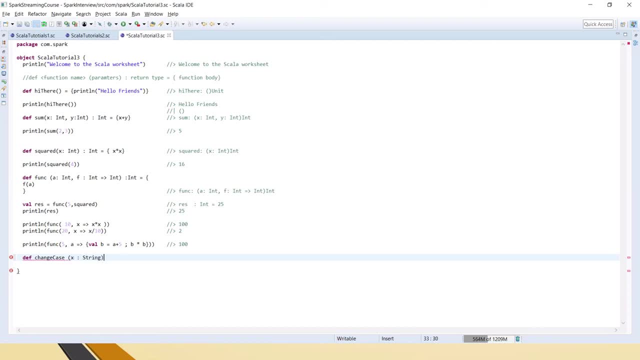 A, And Let's Take A String As Input And Let's Send String As Output Equal To And In The Curly Braces Mention As X. 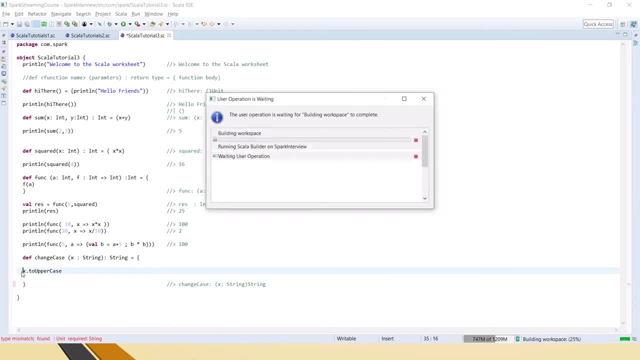 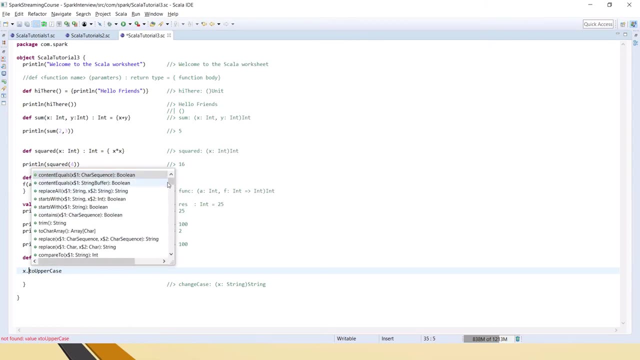 Dot To Uppercase. Okay, You Can Put Dot And Control Enter. It Will Show You Lot Of Function. You Can Use Any Of This. 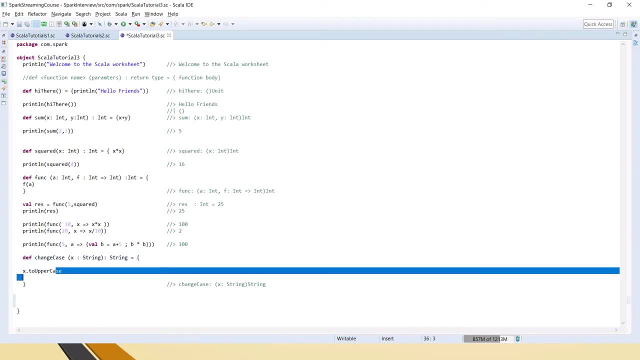 And Try Out On Your Own, Okay, So What We Have Done, We Will Say: Change Case. Which Is This Function? Name Here This Function: We. 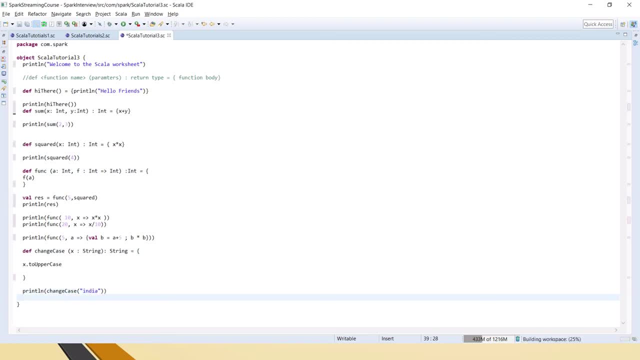 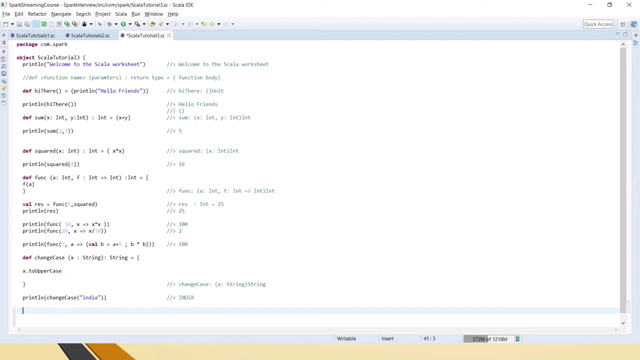 Will Pass It Here And We Will Pass Some Input String, Because That Is So We Have Done Integer Operation And Also We Have Done With. 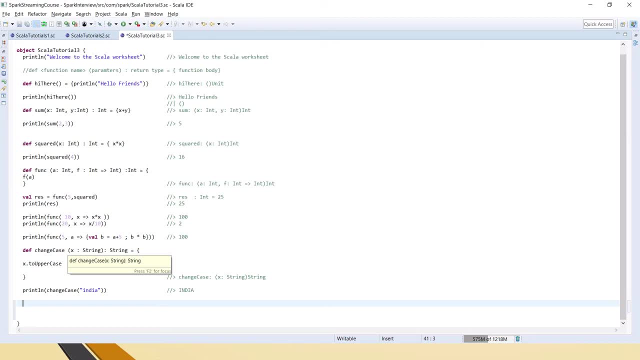 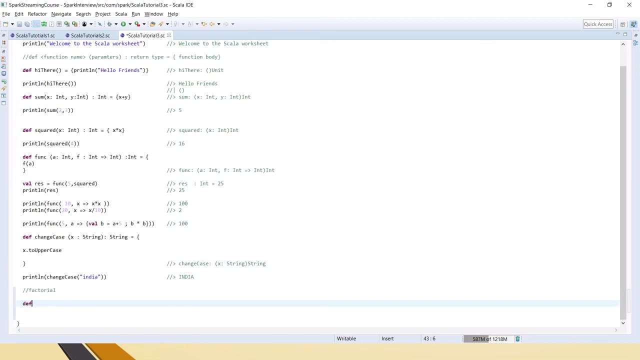 The String Operation. Similarly We Can Do. We Can Use Flow, Double Or Any Kind Of Operations That You Will Understand. What Is The Usually What? 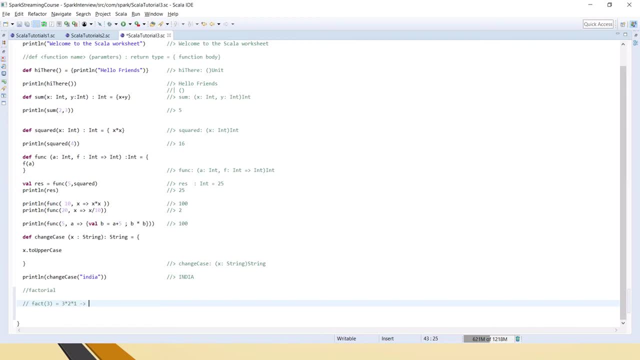 Is The Factorial You All Know Right. A Factorial Of Three Equal To Three, Into Two, Into One Means. If So, That's How The 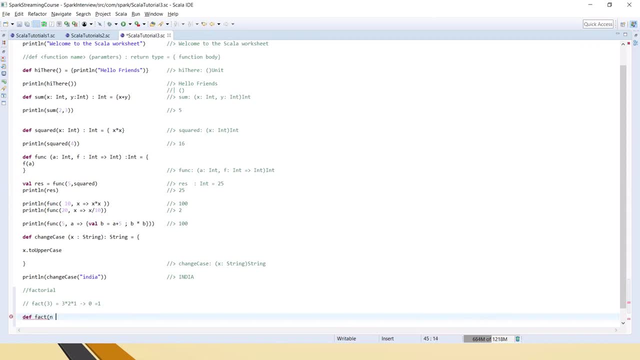 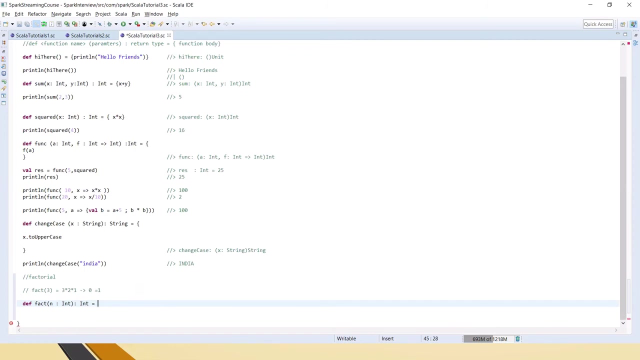 Factorial Is Calculated. So Let's Write A Simple Function For That. So Fact I'm Taking, And We Have To Pass One Integer Right. So 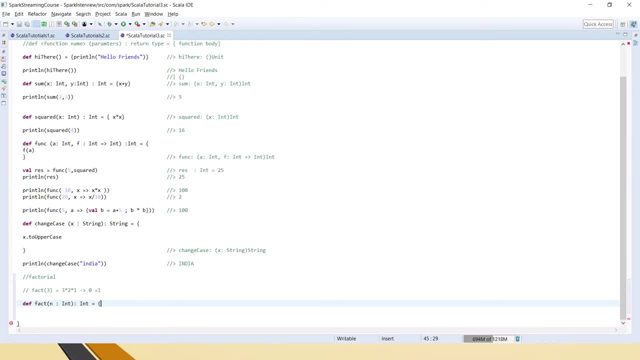 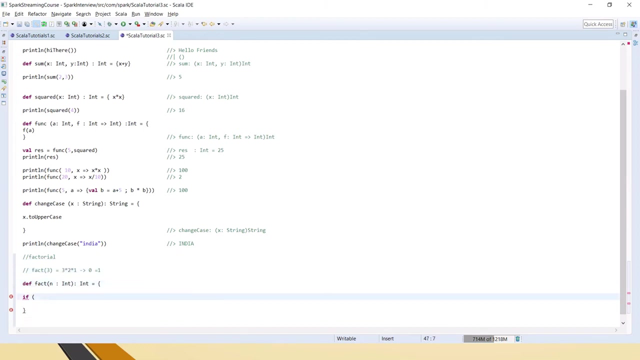 For I'm Giving The Integer Here. Okay, So Now Inside The Braces If We Have To. As I Said, For For Zero Or One Equal. 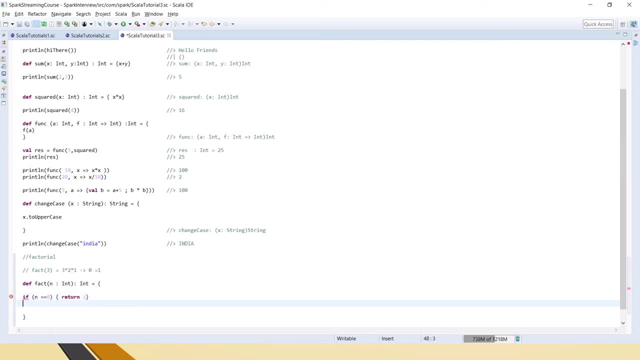 To. It Will Be One. We Have Closed Everything Right. Okay, Else? If It Is, It Is Not Zero, Then Return N Into See How Many. 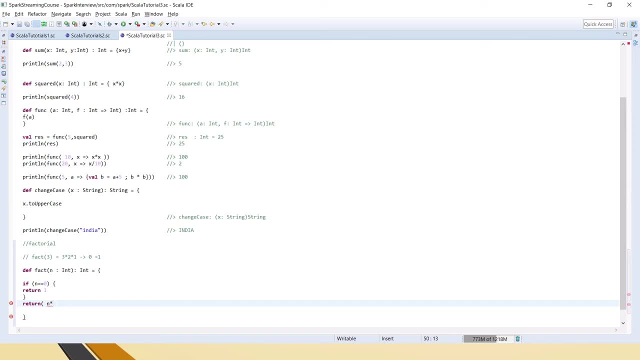 Times. So That's Why I'm Saying That, As To The Same Function We Have To Call Then Only Multiple Times, If We Do Recursively.